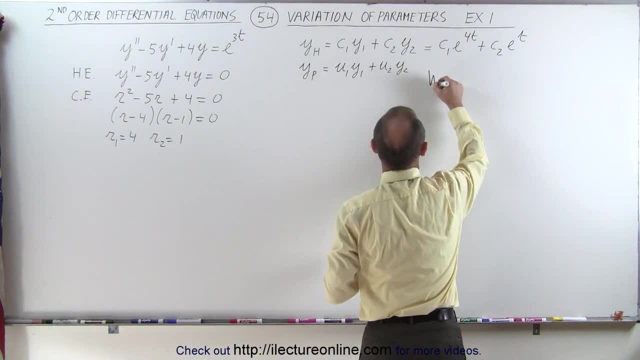 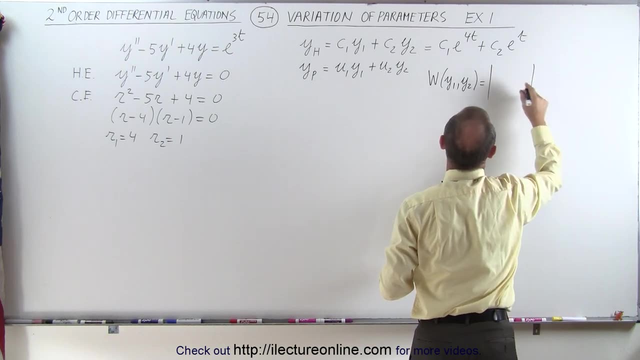 the Wronskian. Let's calculate the Wronskian. So the Wronskian of y1 and y2 is equal to the determinant of y1 and y2, which are right here. that would be e to the 4t and e to the t. 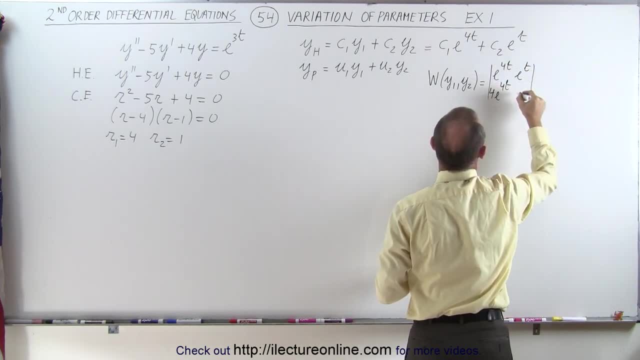 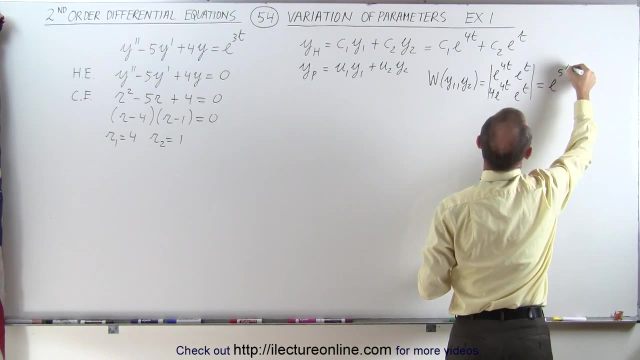 derivative of those, which is 4 e to the 4 t and e to the t, that becomes the product of those two, which is e to the 5 t, minus the product of those two, which is 4 e to the 5 t, which means you have: 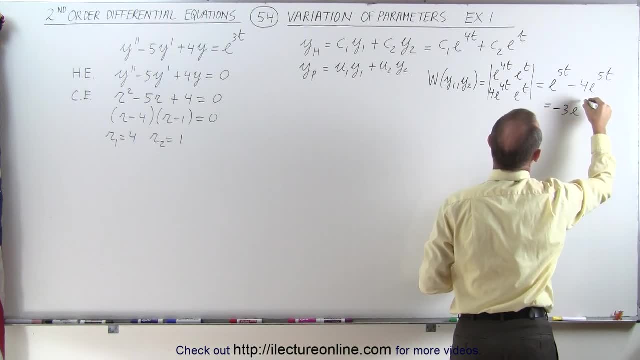 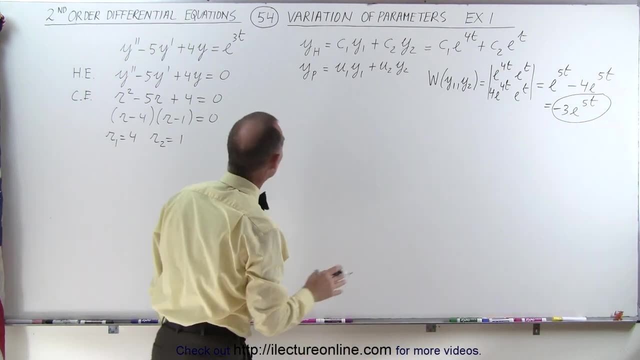 one of those minus four that becomes minus three. e to the five t which is the wronskian of y1 and y2. that comes in handy, because next what we're going to do is try to find u1 and u2. if you remember the 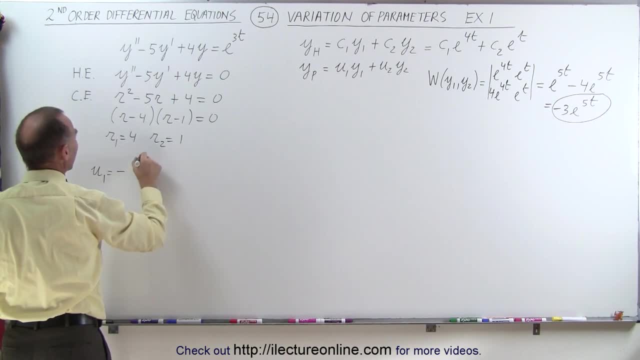 equation u1 was equal to the negative of the integral of y2 times g of t, dt divided by the wronskian of y1 and y2. so plug in what we have. this is negative the integral of y2, which is e to the t. 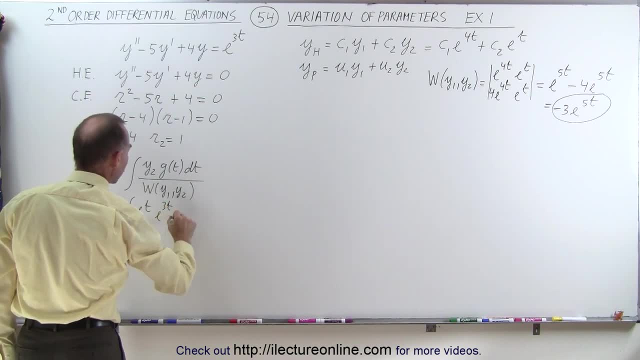 g of t, which is e to the 3 t, dt divided by the wronskian, which is minus 3 e to the 5 t, this is equal to the negatives. will cancel out. i can pull out a: 1 over 3 times the integral of e to the 4 t. 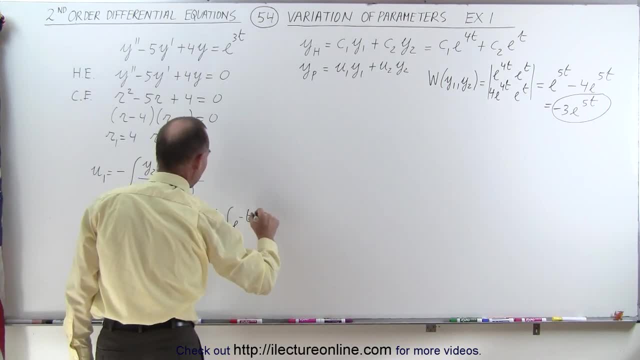 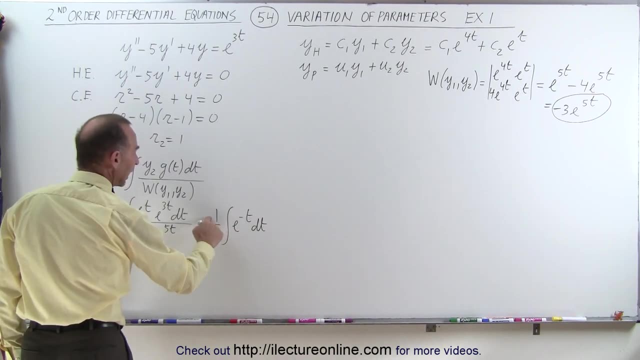 divided by e to the 5 t, which is e to the negative t, dt, and if we integrate that we can say that u1 is equal to. of course we're going to need a negative 1 that becomes negative one-third e to the negative t, plus a constant of integration. 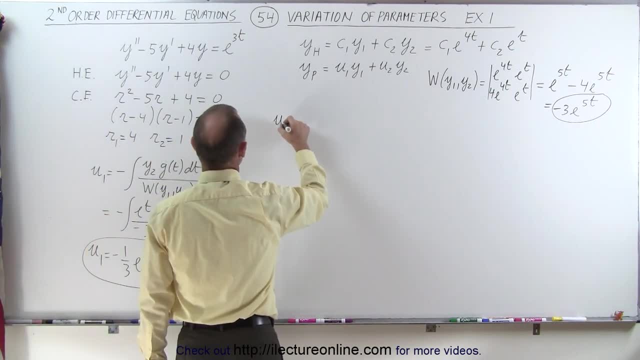 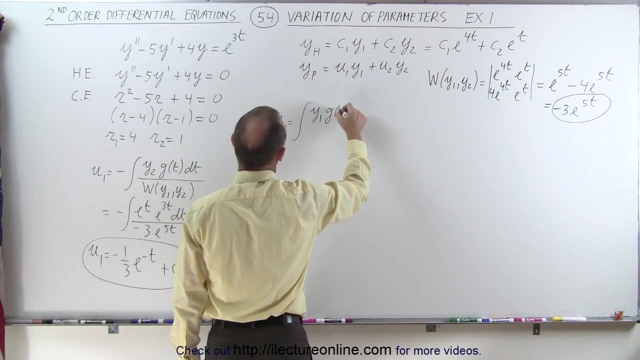 now we can do the same for u2. u2 is going to be equal to the positive of the integral of y1 times g of t dt divided by the wronskian of y1 and y2, which is equal to. oh yeah, i have a dt which is equal to the integral of y1, which is e to the 4t. 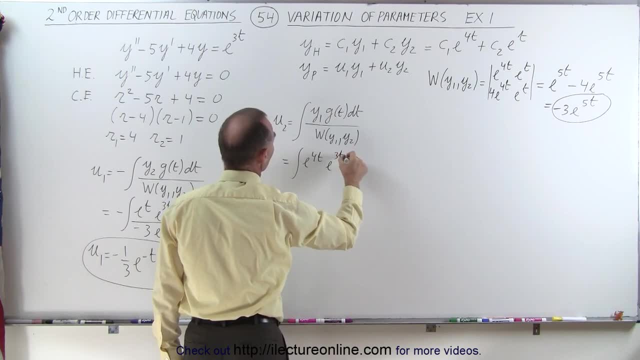 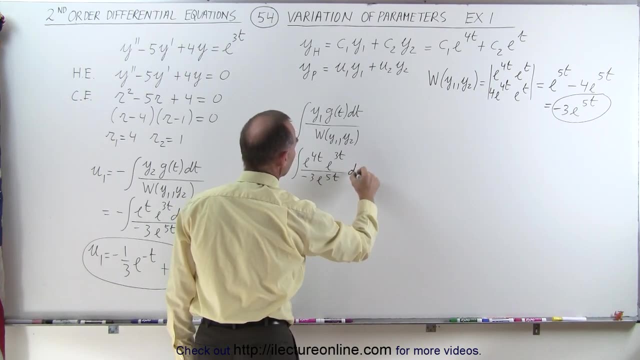 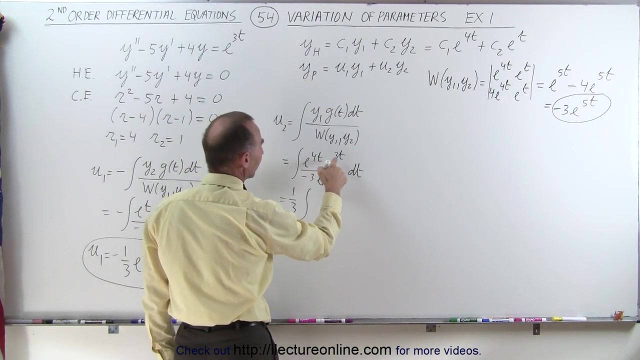 g of t, which is e to the 3t, divided by the wronskian, which is minus 3 e to the 5t. of course we're going to need dt. i can pull out a negative 1 over 3 times the integral of e to the 7t divided. 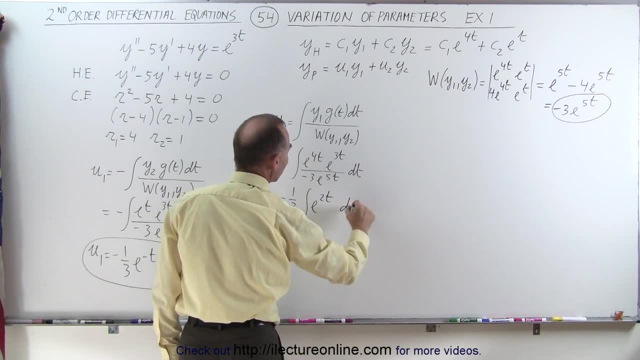 by e to the 5t, which is e to the 2t, divided by e to the 7t, divided by e to the 5t, which is e to the 2t. dt. of course, integrate that we're going to need a 2d t. 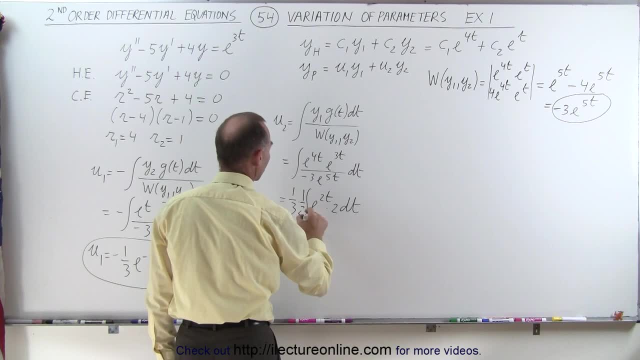 and we need a 1 over 2 to compensate for multiplying this times 2. and do i still have my negative here? i lost my negative, so make sure i have a negative in there because there was a negative there. so this becomes equal to negative 1 over 6 times e to the 2t. 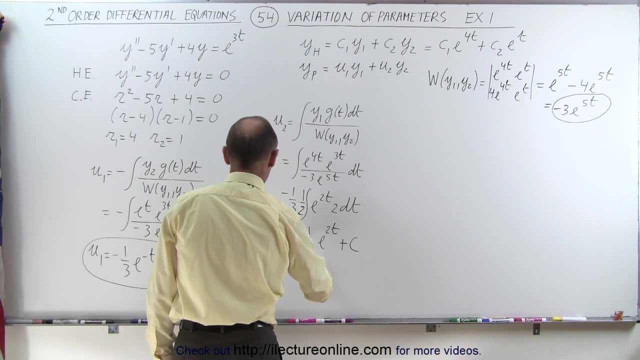 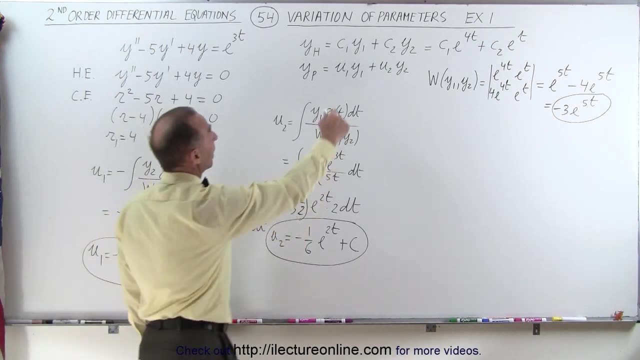 plus a constant of integration, and so that would be equal to u1 over 6 plot e to the 2t plus a U2.. So now that I have U1 and U2, I can go ahead and plug that into my particular solution. 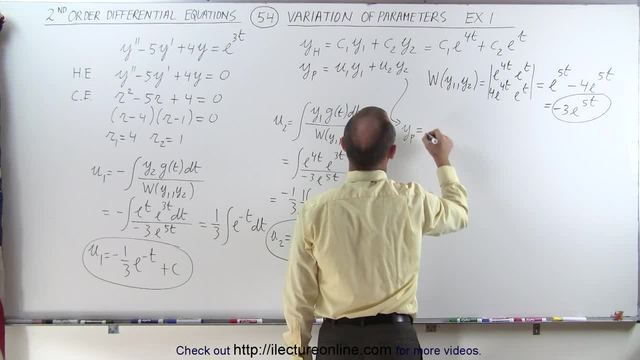 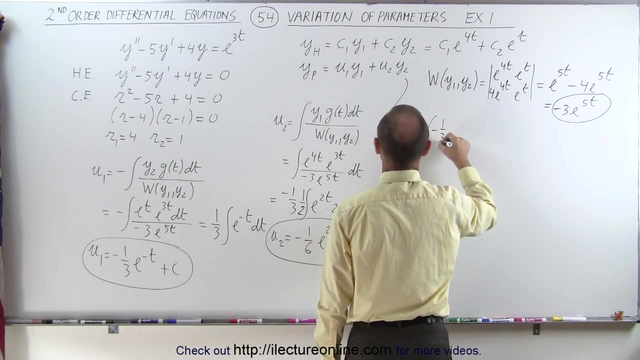 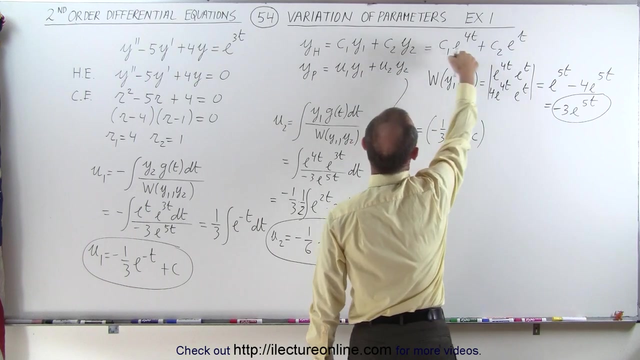 equation. So I have the particular solution for the differential equation is equal to U1,, which is minus 1 over 3, e to the negative t plus the constant of integration times, y1, and y1 is e to the 4t plus U2,. 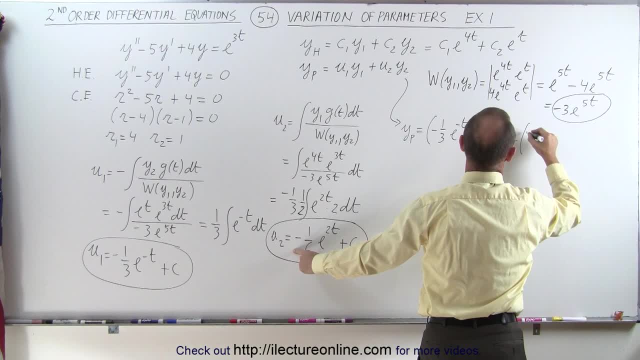 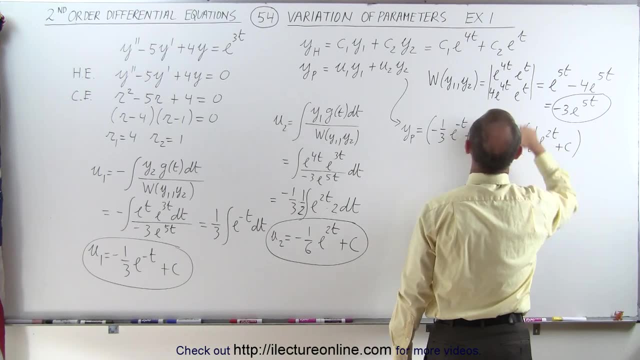 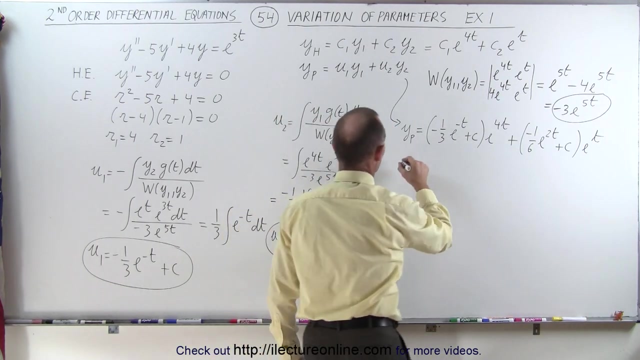 which is minus 1 over 6, e to the 2t, plus the constant of integration times, y2,, which is e to the t. Now we just need to clean it up a little to see what happens. So y particular is equal to: 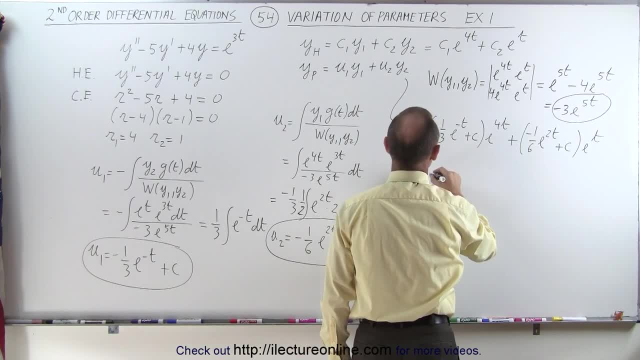 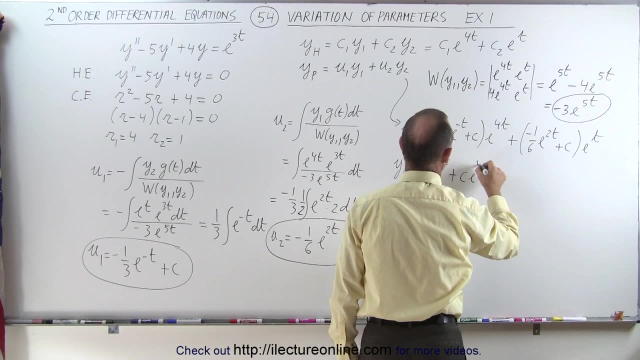 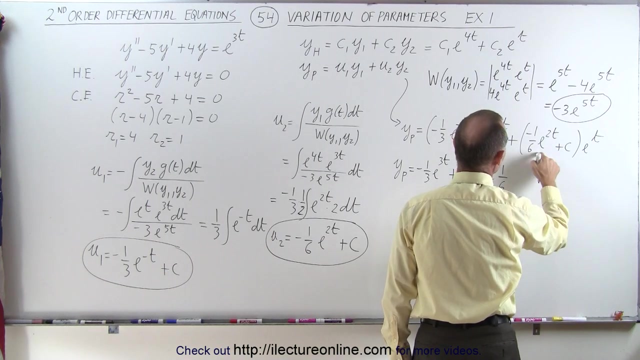 multiplying this times this, that would be e to the 3t, so minus 1 third e to the 3t, plus a constant times e to the 4t. And then here we have a minus minus 1 over 6 e to the 2t times e to the t, which is: 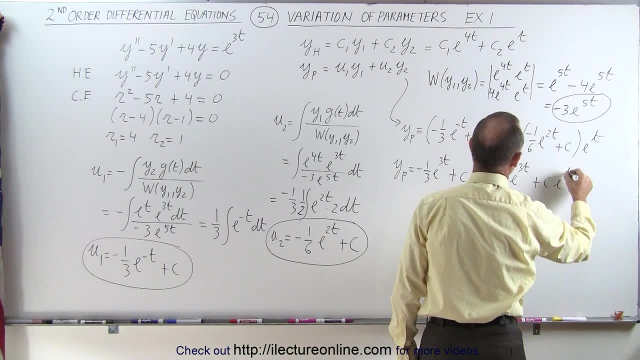 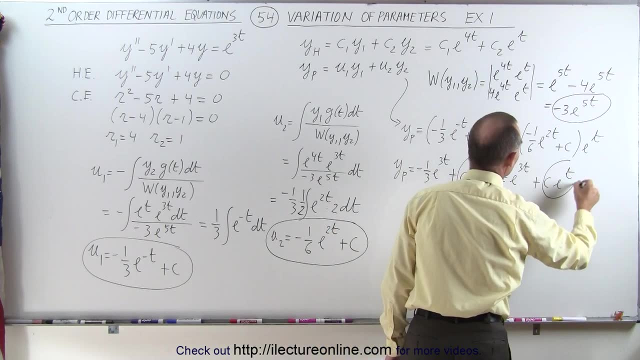 e to the 3t, plus a constant times e to the t. Now take a look at these two terms right here: c? e to the 4t and c? e to the t, Since our homogeneous solution already has those two functions in it. 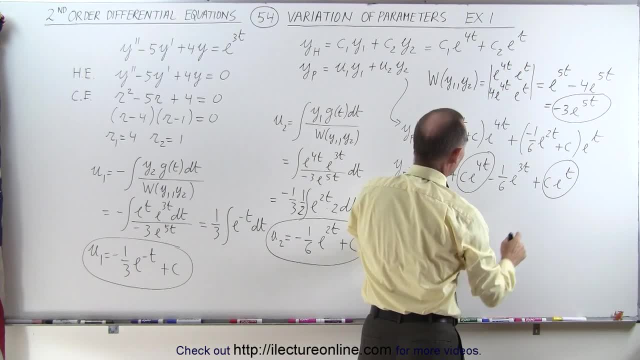 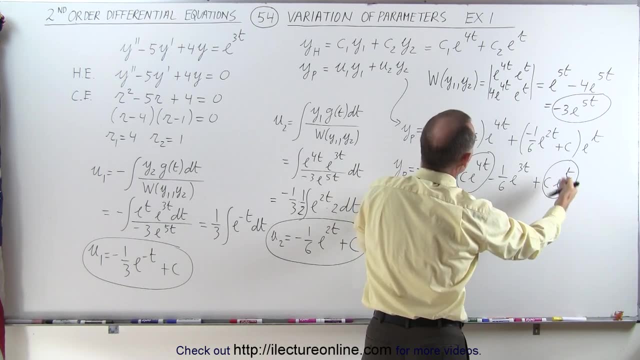 with some arbitrary constants- c1 and c2, if we then add these two terms to that, we're still going to get e to the 4t times some constant, and e to the t times some constant. so these will get absorbed in the homogeneous part. 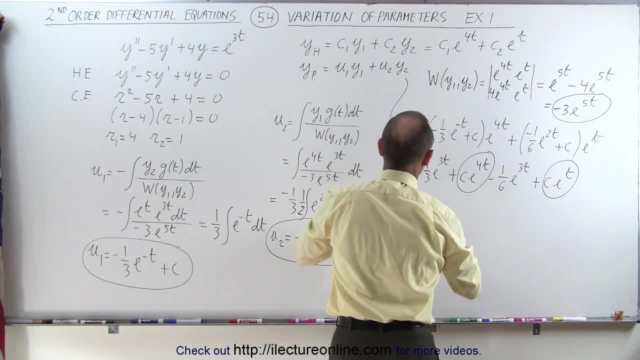 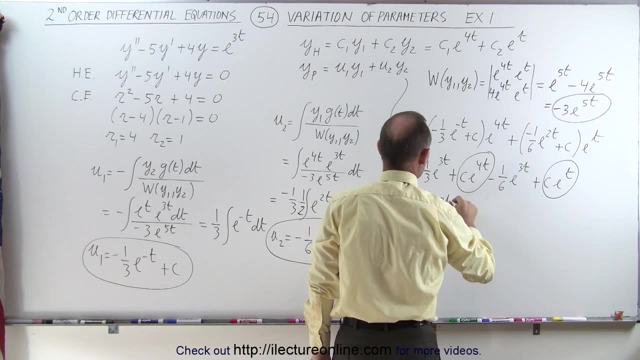 of the solution, so we don't have to worry about those. That means the particular part of the solution becomes as follows: y particular is going to be equal to minus 1 third e to the 3t, minus 1 sixth e to the 3t. 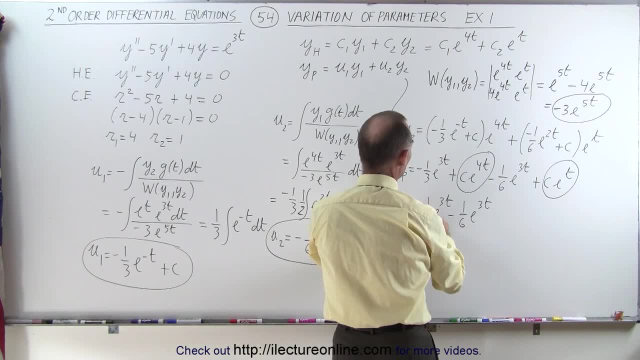 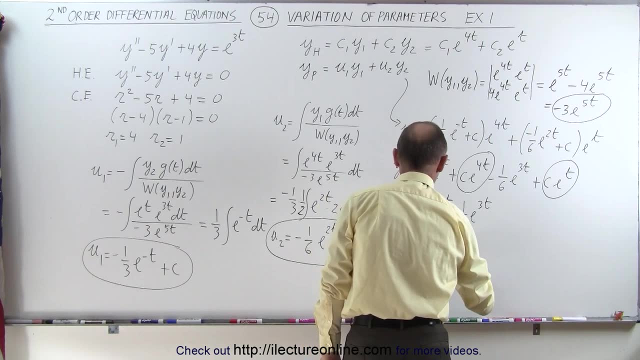 Of course, when we combine common denominators, that is minus 2, sixth minus 1, sixth, that's minus 3, sixth, or y particular is equal to minus 1 half e to the 3t, And that is the exact same particular solution. 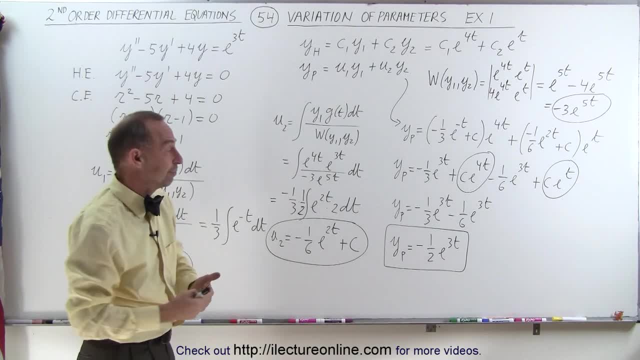 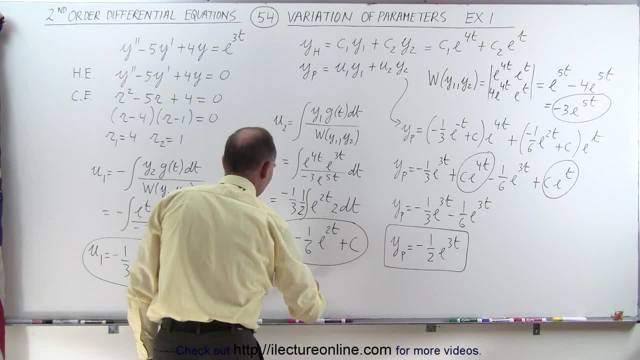 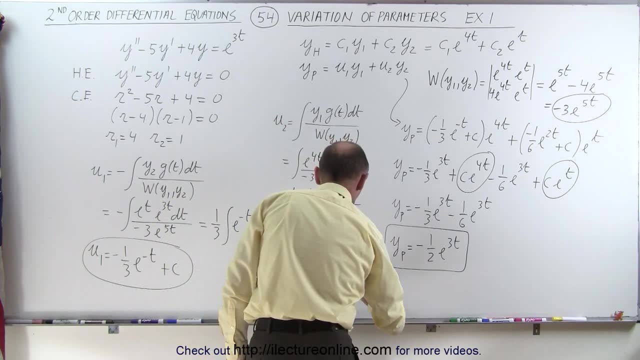 we're going to get you know. we're going to get you know. but the solution y is a function of t, which is the sum of the homogeneous part plus the particular part of the solution. so that would be equal to c1e to the 4t. 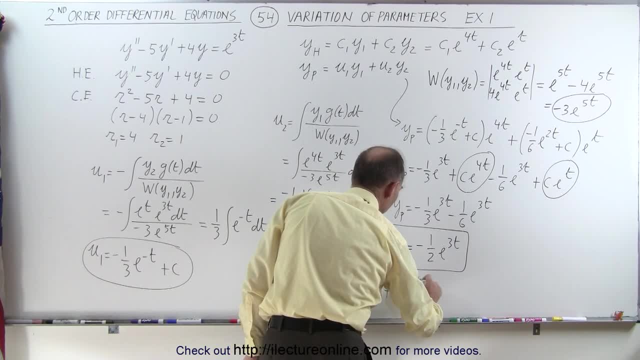 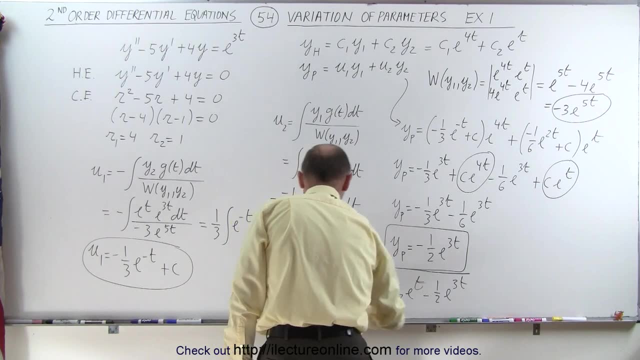 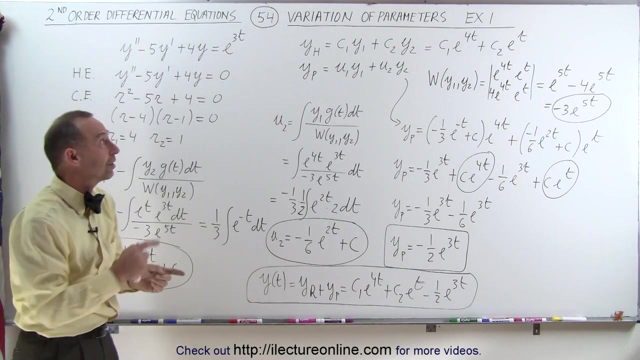 plus c2e to the t, minus 1 half e to the 3t for the particular part of the solution. and this gives you the general solution of this original homogeneous differential equation, but in this case, In this case we use the method called variation of parameters instead of the undetermined coefficient method.